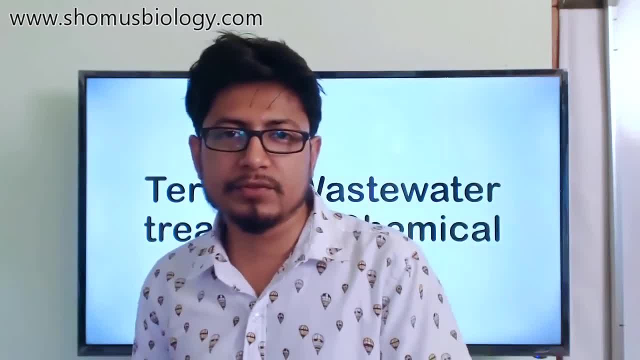 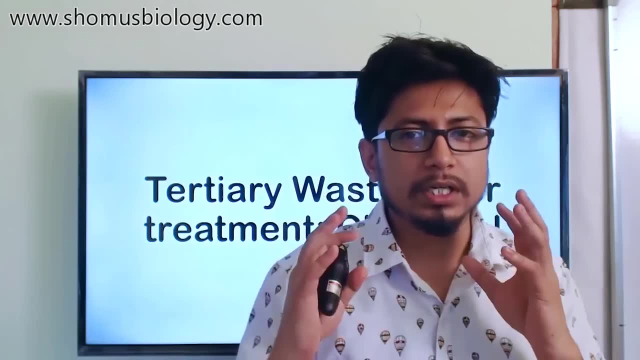 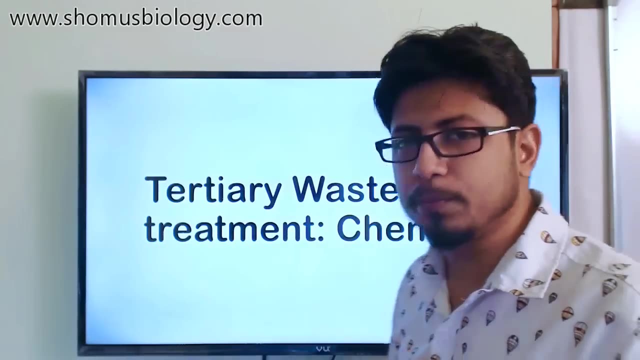 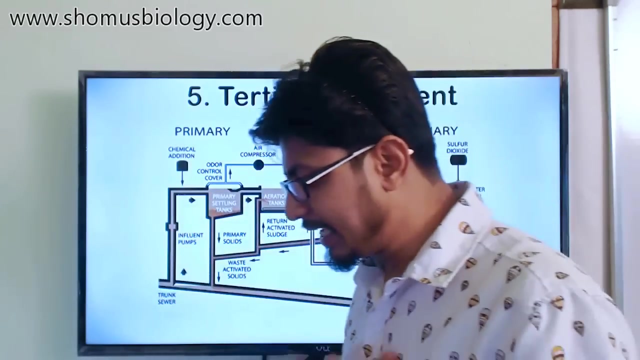 waste water treatment When the water is already being treated in the secondary water clarifier, so secondary sedimentation tank- the effluent is then transported to the tertiary wastewater treatment facility. In the tertiary wastewater treatment facility we use chemical agents to purify the water, And in the tertiary treatment facility the chemical agents that we use is mostly gaseous material like chlorine ozone. So if you look at this picture with all the overall 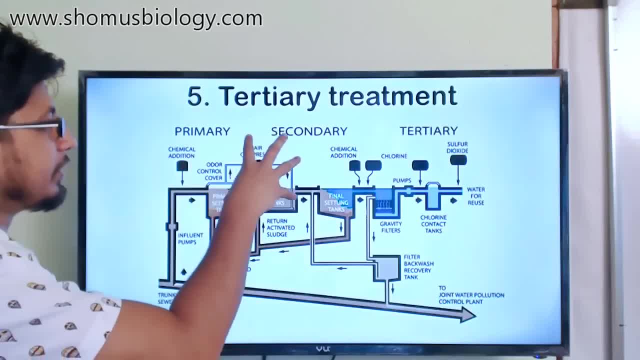 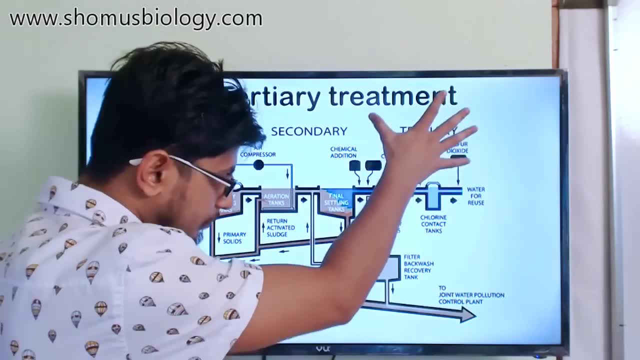 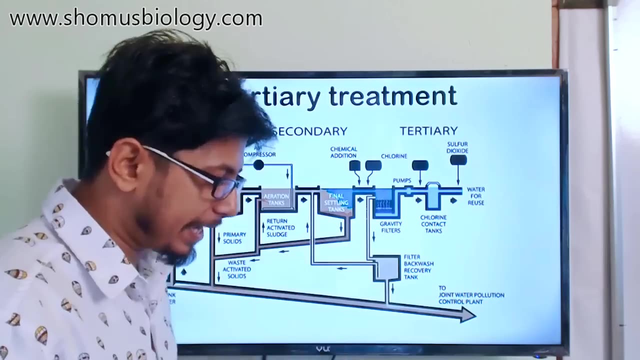 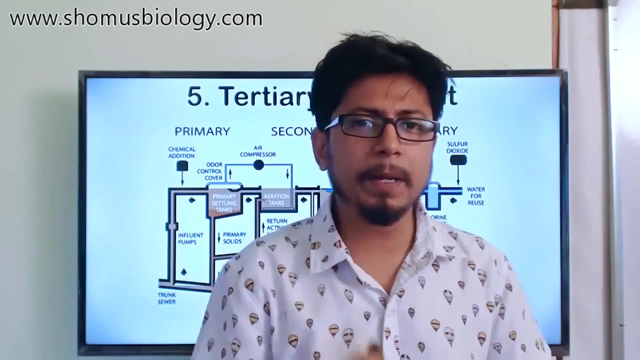 steps. we've talked about this preliminary treatment, the secondary treatment, primary treatment, secondary treatment And, after the secondary treatment is done, when the final effluent is transported into the tertiary treatment. it's all about modifying that effluent and utilizing chemicals to kill any of the microorganisms that may be present in that water Because, remember, just before this tertiary treatment, in the secondary wastewater treatment, we use microorganisms. 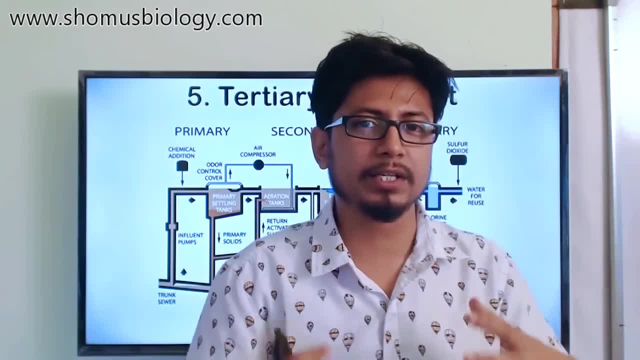 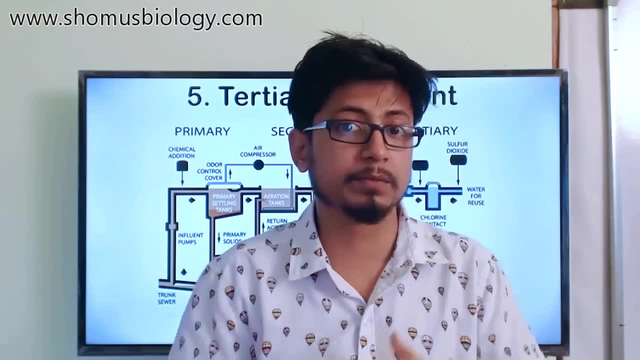 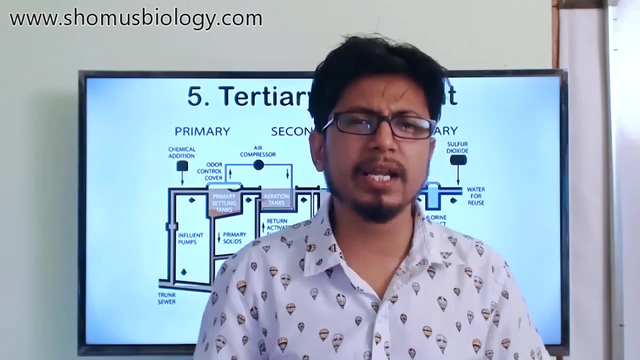 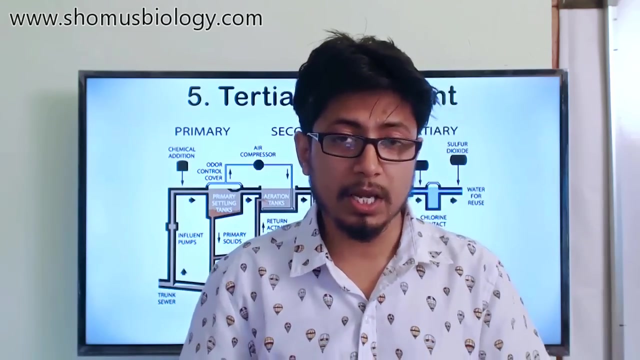 to take out all the organic, destroy the organic materials from the wastewater treatment And they use it to grow themselves And generally, that's how the biofilm of microorganisms are produced Now, as a result of which we can assume that this effluent may contain a huge load of microorganisms. But we cannot drink that water filled with that huge amount of microorganisms because maybe some of them are pathogens, Maybe some of them can harm us in many different ways. 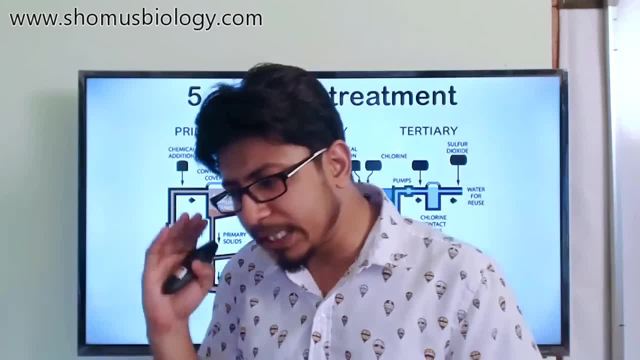 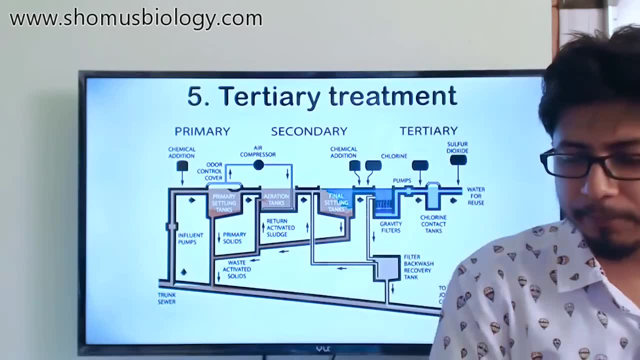 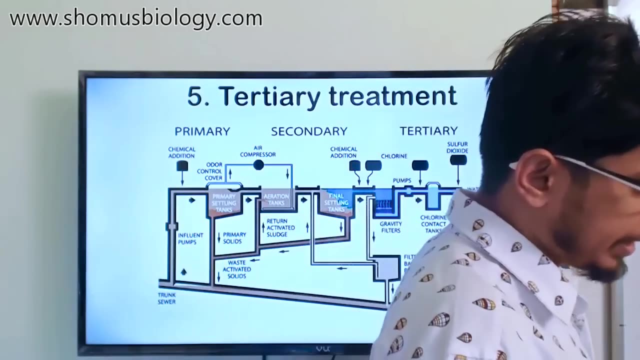 modes. so that's why it's very important key any of those living microorganisms that is present there. so what we do, our target, is to kill them. so because the job of the microorganisms are already done, we don't need them anymore. so we use chemical agents to kill it. and what kind of chemical agents we can use to? 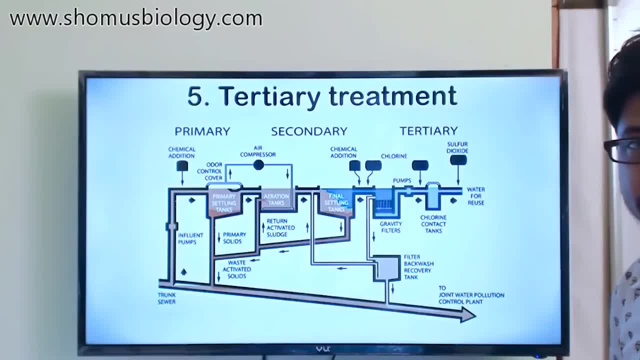 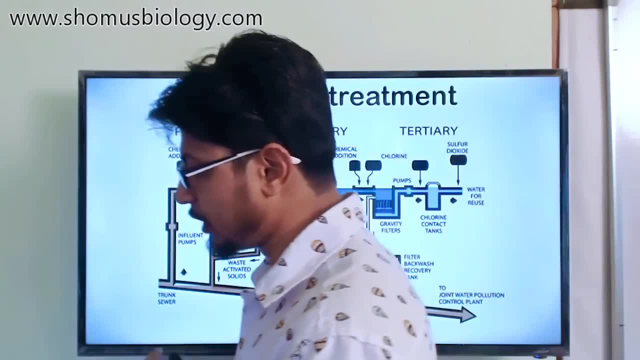 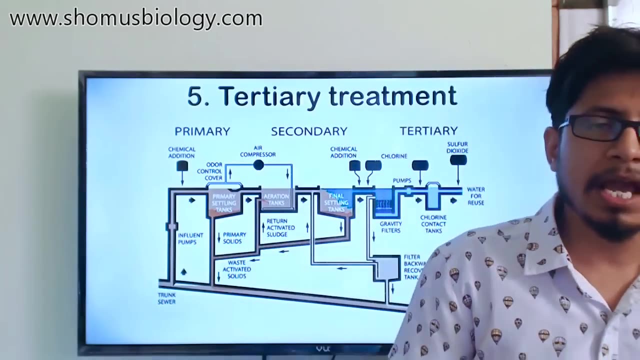 kill microorganisms. we can use chlorine- okay, we can use ozone gas to kill it. so chlorine is most commonly used as a tertiary worst water treatment chemical agent and chlorines are used mostly as a gaseous form. there are huge giant cylinders and those giant cylinders are filled with chlorine gas. that can be a 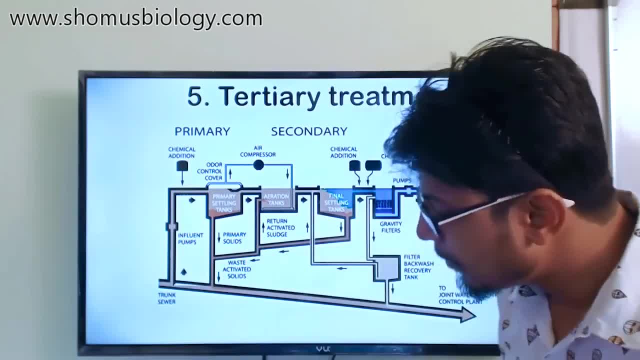 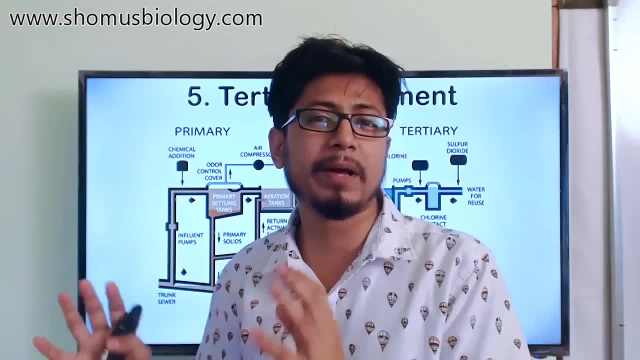 one-ton cylinder, or even hundred pound, two hundred pound cylinders, depending upon that. all can use liquid chlorine, or people can use tablet chlorine that will do the same, but in the worst water treatment management facilities we use gaseous chlorine, and the gaseous chlorine is. 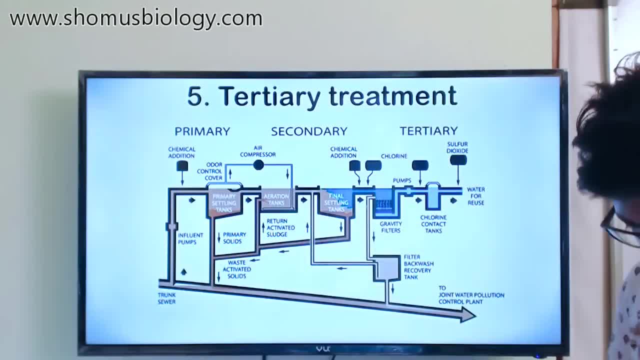 inserted in the gaseous chlorine and the gaseous chlorine is inserted in the into the gravity filters. now remember the final step. the final step includes this. to this: this tertiary treatment includes the two different mechanical structures. one is the air mediated gravity filter, another one is the chlorine. 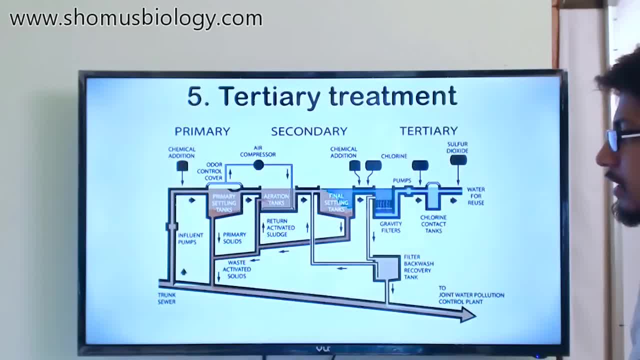 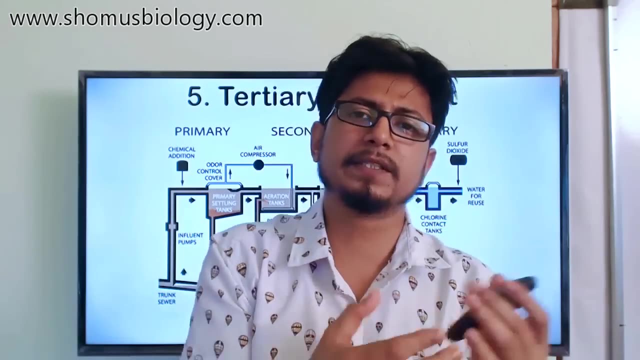 chamber. so the very first step is with the gravity filters. this is where all the effluent of this that's coming from the secondary sedimentation tank transports into the gravity filter, and the gravity filter is like a filter. that filter separates any other, any other particles that are present in that water from the 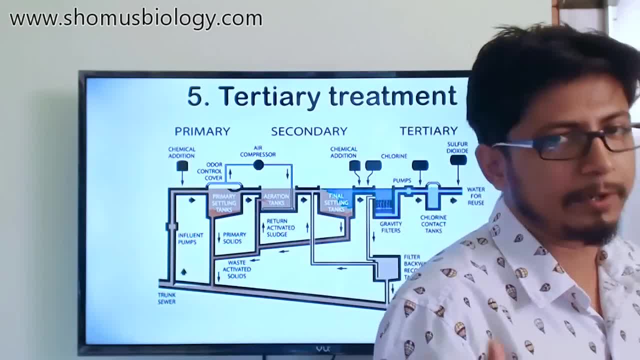 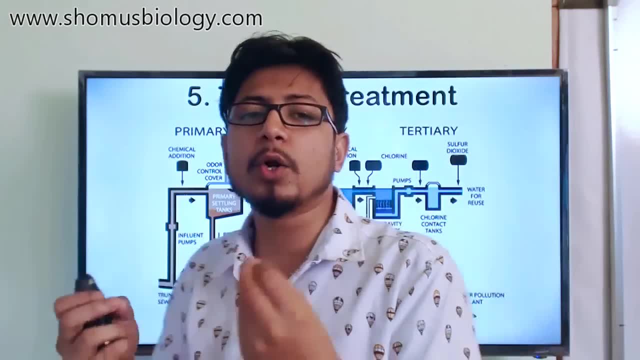 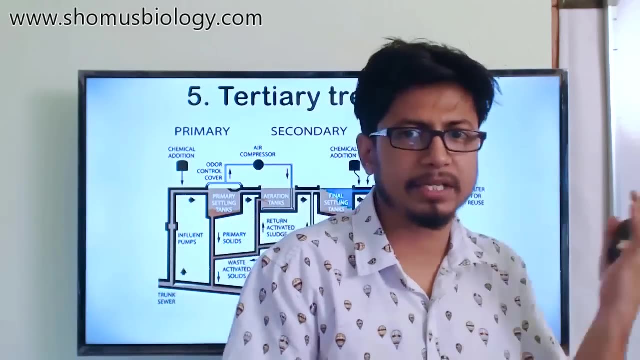 liquid as very fine filter that are produced. sometimes people can also use here the ultra membrane filter. okay, so that is going to separate any other microorganisms either supplied, like large biofilms which are produced by the, by the next line layers which are produced, which can clearly separated. 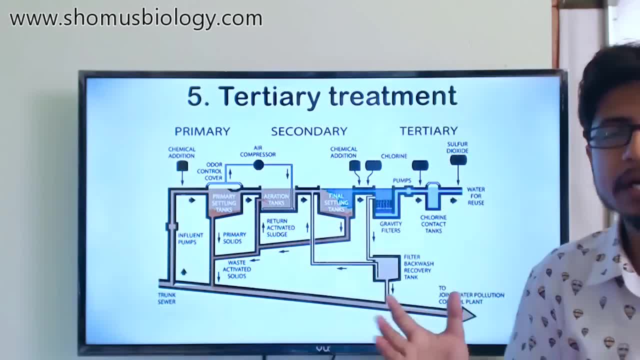 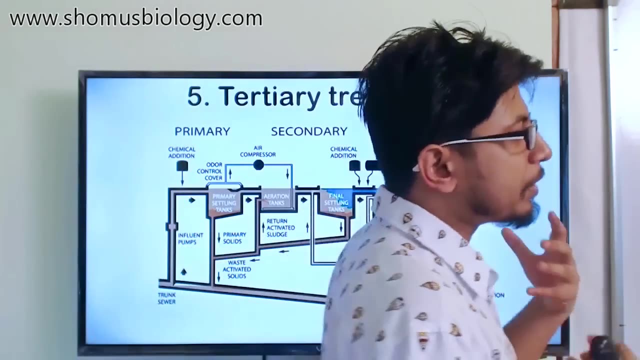 microorganisms, you know, which are present as a, as a form, can be separated with the help of this gravity filters. but after this filtration is done, still they may have some bacteria, because bacteria are very tiny and we don't use that amount of tiny filters in this gravitational filter. chamber gravitational filter. 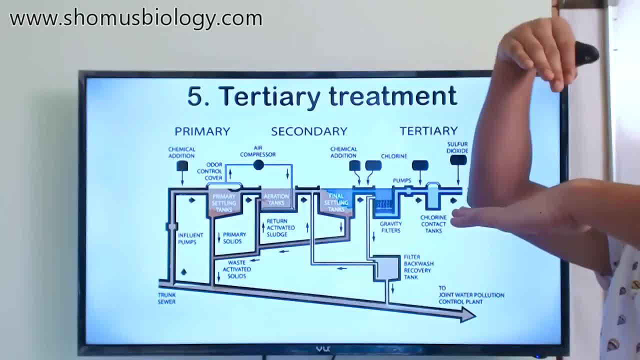 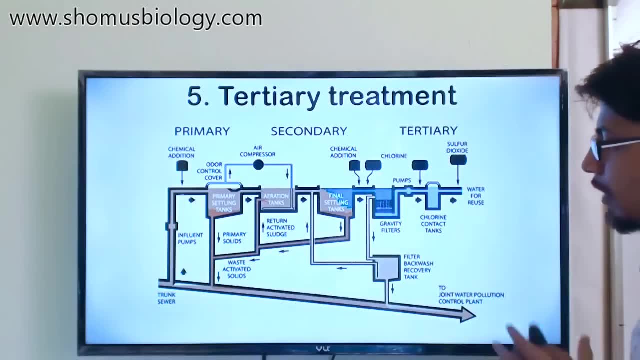 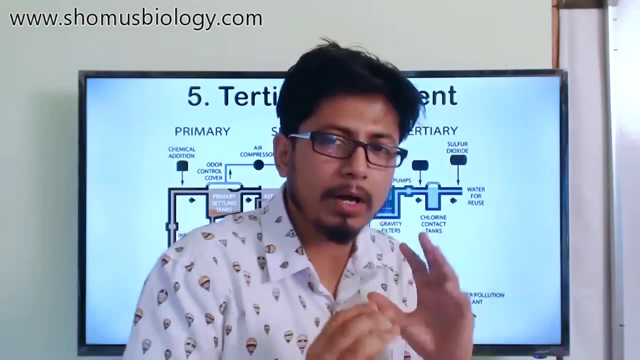 works by, by utilizing the filters, and water is flowing down through the filter into the bottom in the collecting chamber. through the chamber, we pumping the influence out to the chlorine tank. in the chlorine tank now any other bacteria which is living, any other protozoa which is still living, can be killed by the chlorine treatment because they will not withstand the amount of chlorine that we use and the chlorine treatment is generally done for a long period of time because, you know, it's not like the higher concentration of the chlorine but it's more time that the microorganism is in contact with the chlorine that can. 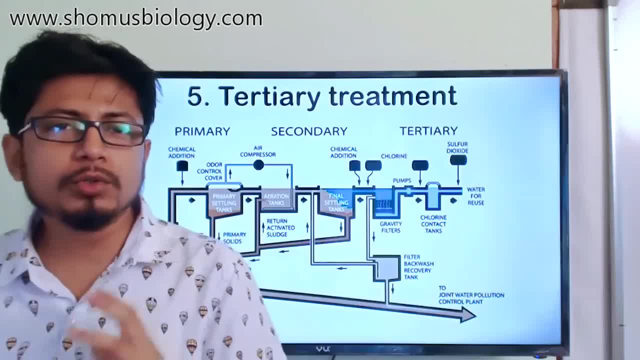 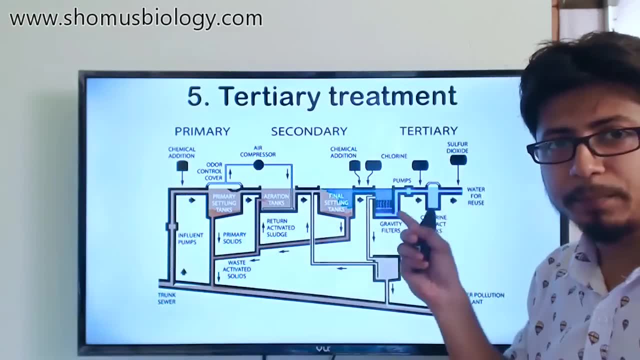 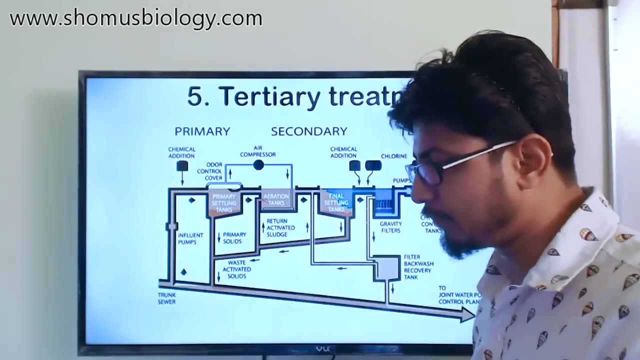 kill them. so that means, while you're using a chlorine treatment, do not think of increasing the concentration of chlorine, because if we increase the concentration of chlorine, that's chlorine is going to be present in the water and that will be harmful for the eltimate discharge water, because the water goes to the stream. the fish can be damaged. 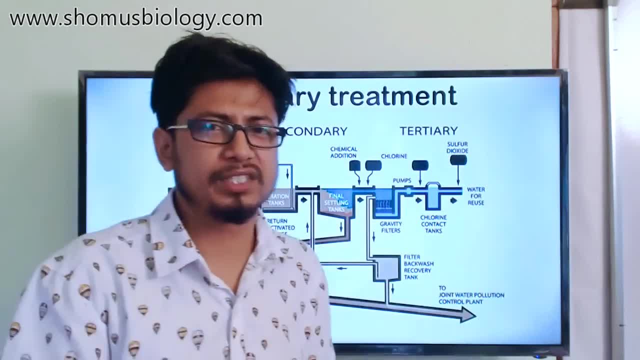 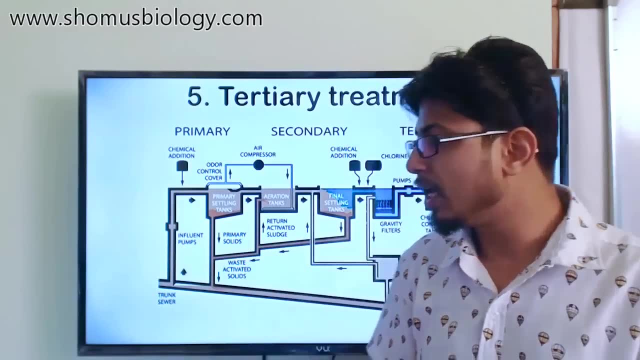 because fishes are much more harmful to chlorine than us, because we can still drink chlorinated water. we can. we can take a tap water is generally chlorinated because our municipality does that- but still a fish cannot withstand that amount of chlorine. that's why it's always prescribed that use a. 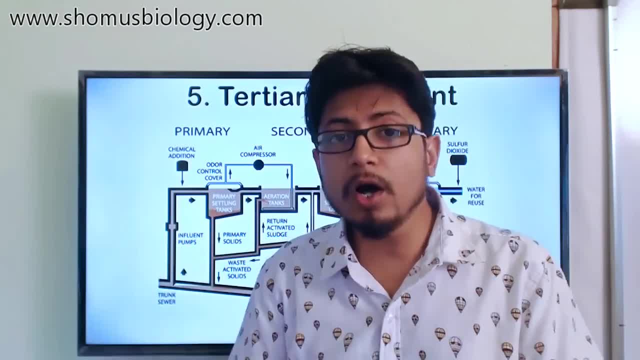 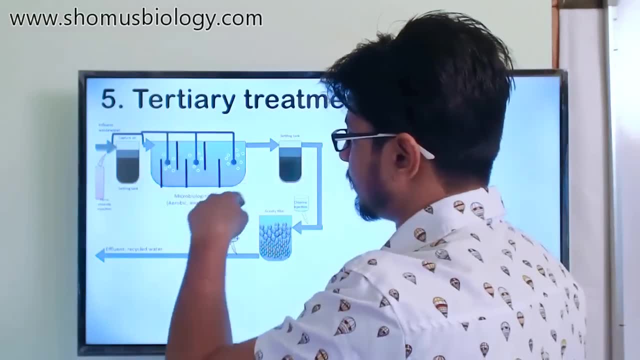 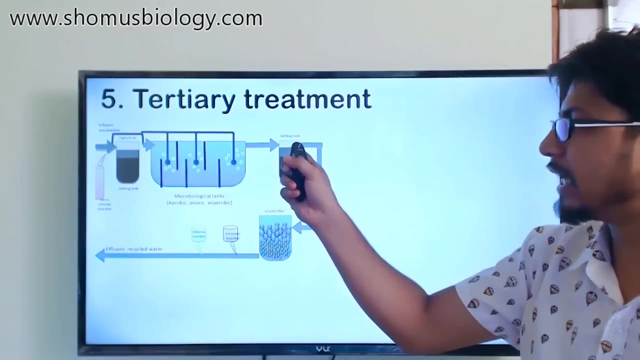 less amount of chlorine, but longer duration of time. the wastewater is in contact with the chlorine tube. So this is what works in these microbiological tanks: the secondary treatment in the settling tank. This is where the gravitational settling takes place, and after that the effluent is collected. to this 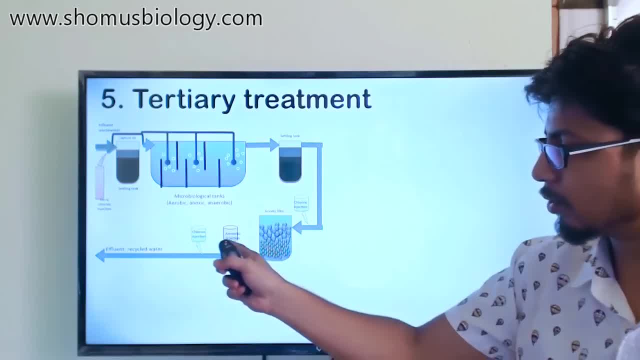 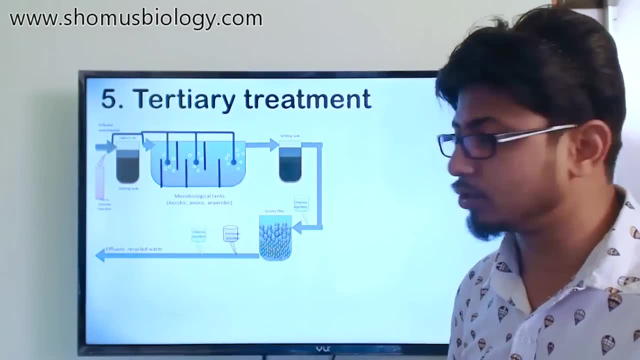 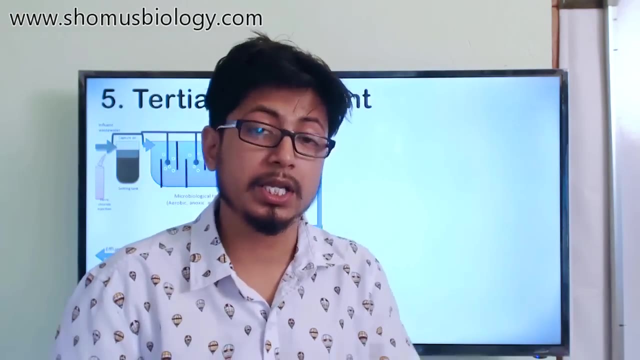 derivative filter, Again another mode of filtration, and finally goes to the chlorine injection. and then, after the chlorine injection, the effluent is recycled. Sometimes, along with the chlorine, ammonia injection is also being mediated before releasing the water. Not only ammonium injection, but also sometimes sulfur dioxide injection is also mandatory. 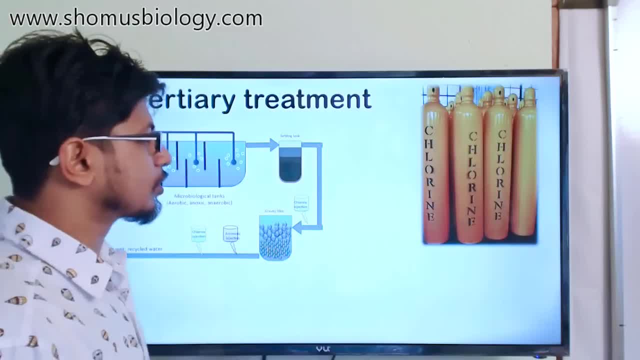 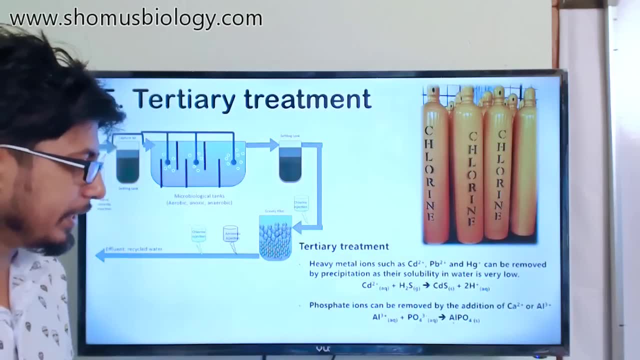 Hydrogen sulfide injection is sometimes mandatory, But mostly we use chlorine for this treatment. So you see, the heavy metals sometimes can be present in the water, like cadmium, lead, mercury And generally cadmium. if we add hydrogen sulfide it's converted to a very low form. 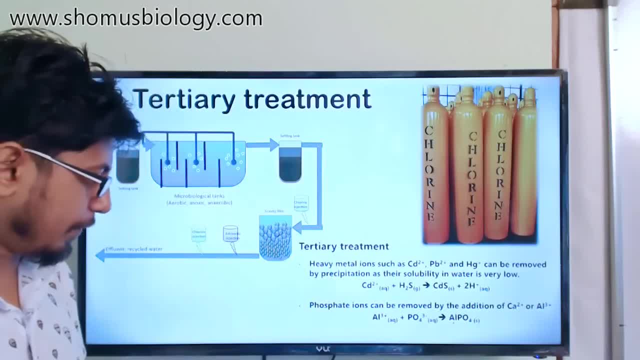 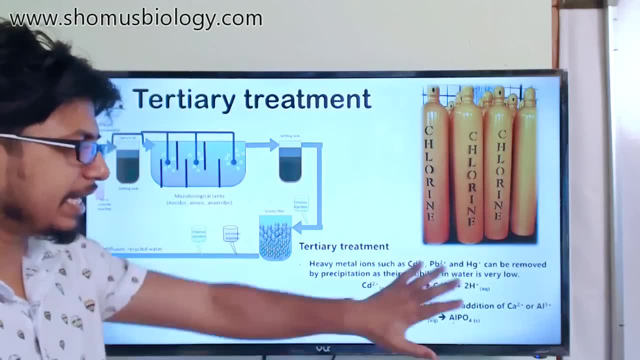 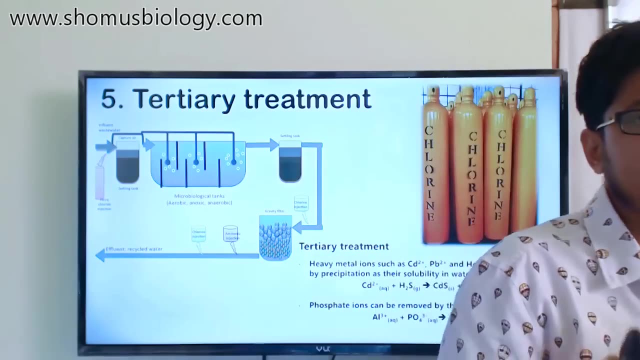 that we can separate from there Very less damaging form. Similarly, phosphor diodes can be removed by adding calcium or aluminium ions in there, So that can be done to separate those heavy metals from the water. Because you know, now the concern is chemical concerns, Because the sewage may. 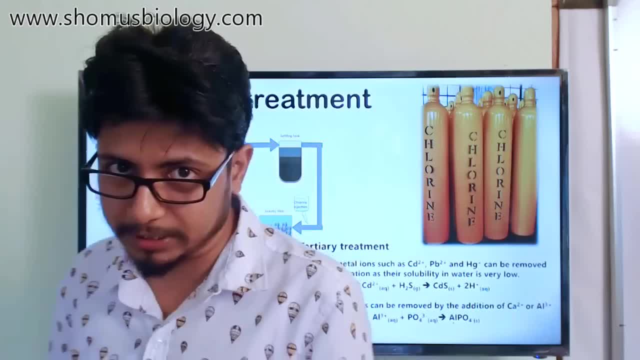 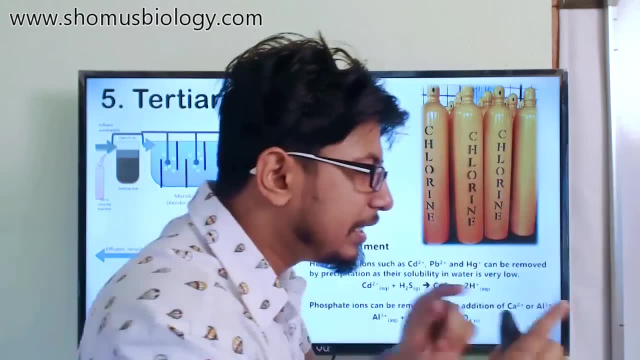 also carry these heavy metals, which may lead to heavy metal toxicity and poisoning. So to prevent that we can do further processes. But our primary target of a tertiary treatment is to kill the microorganisms that are living. So that's why we first use the gravity filter to separate any other debris, any other. 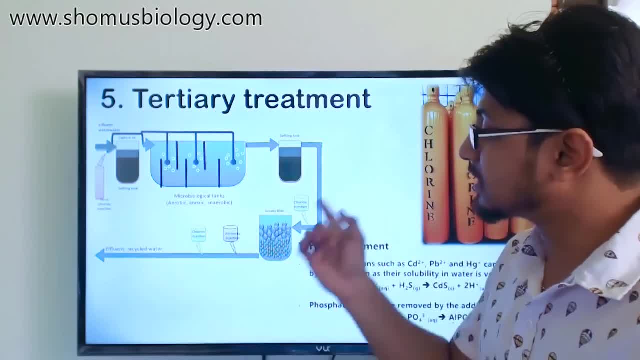 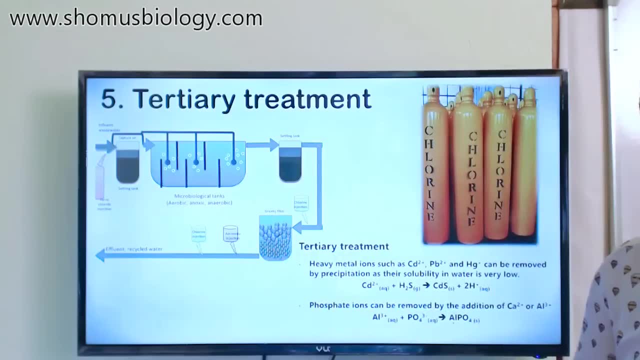 bacterial microorganisms, body portions from the effluent, And still, if in the effluent we have a living bacteria or protozoa or fungi, that can be killed by the chlorine, And chlorine is generally ingested as a gaseous form. So that's the overall process of tertiary treatment. 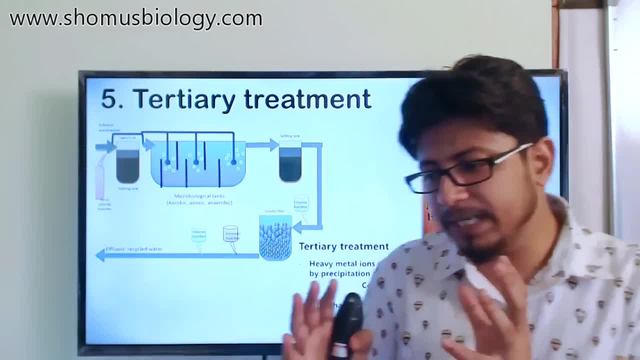 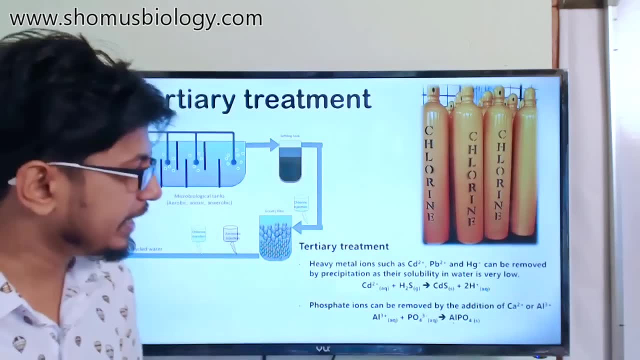 that we generally do So. remember, as I mentioned, that we simply allow the water to be in contact with this chlorine cylinder, or chlorine gas, for a longer period of time, And thus it ensures better safety of the water, because it will kill it And SO2 is also sometimes used to. 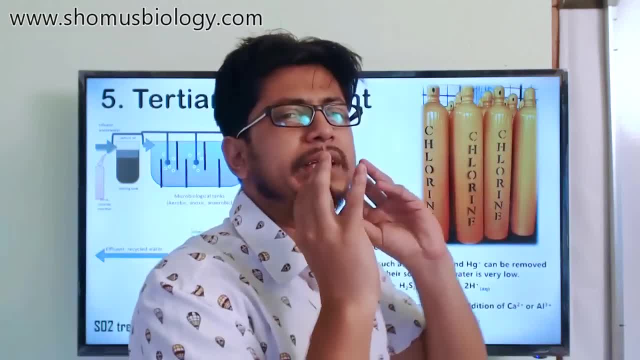 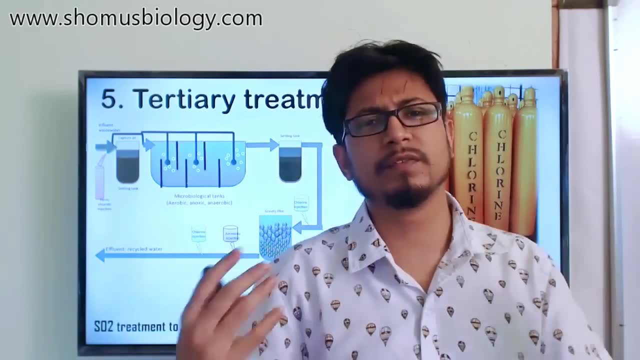 reduce the chlorine in the water. Now remember at the end: we know we use chlorine And we know if we allow chlorine to diffuse in the water for 3-4 hours, We know that most of the bacteria, in fact all of the bacteria, will be dead. 99.9% bacteria are gone. 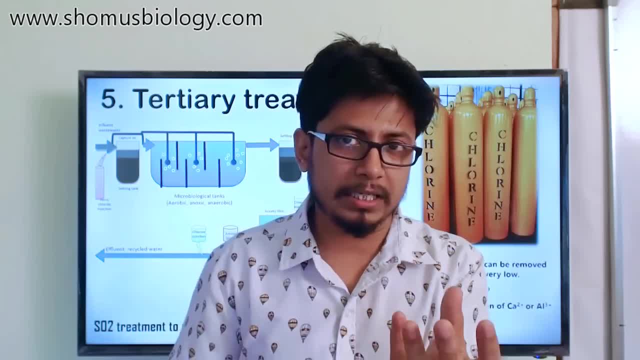 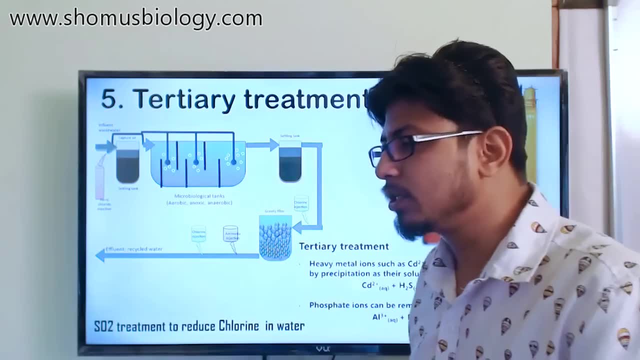 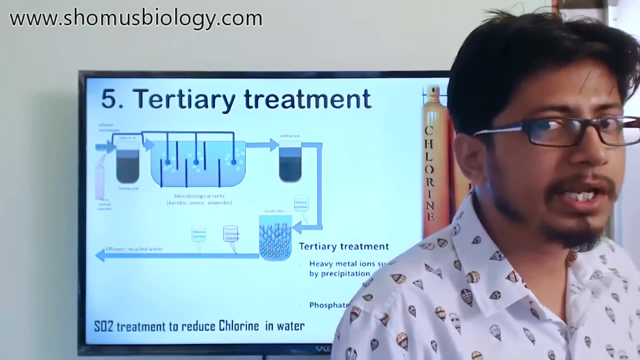 But now the question is: chlorine is there in the water And the chlorine can damage the water ecosystem. So what to do To reduce the chlorine? sometimes we can use chlorine filter or we can see a washing filter. It's expensive. That's why most of the wastewater treatment plants do not use it. Instead, what they use is sulfur dioxide gas. 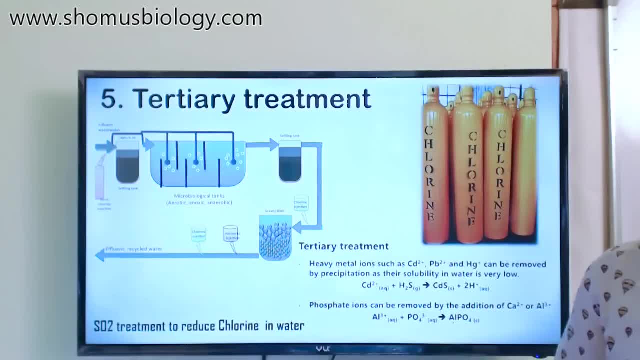 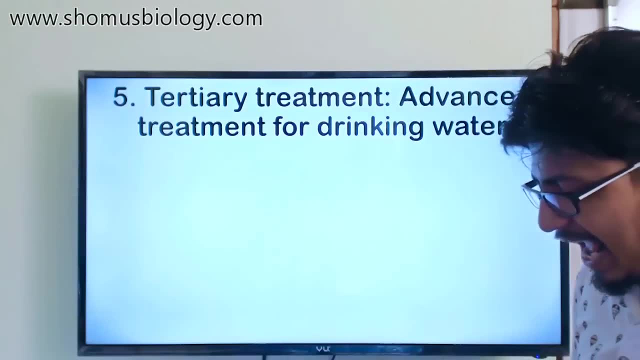 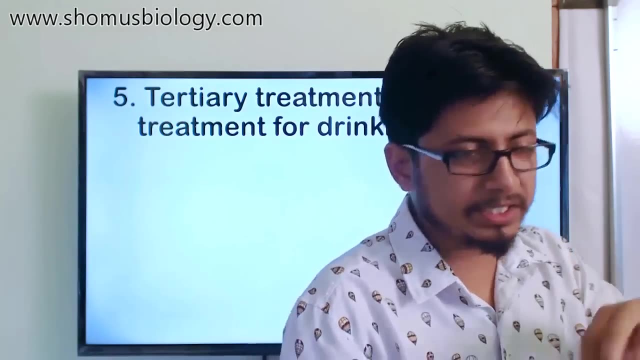 When they use sulfur dioxide gas. the sulfur dioxide gas neutralizes the effect of chlorine in the water And then we reduce the water into the water stream And in few occasions. not all the wastewater treatment facility produces the water for drinking. They simply produce the water for portable water purpose, For the household water activities. 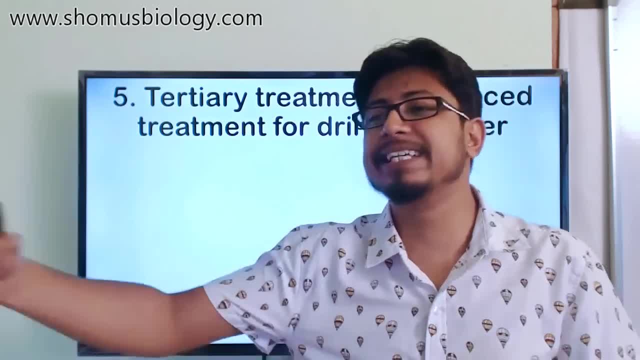 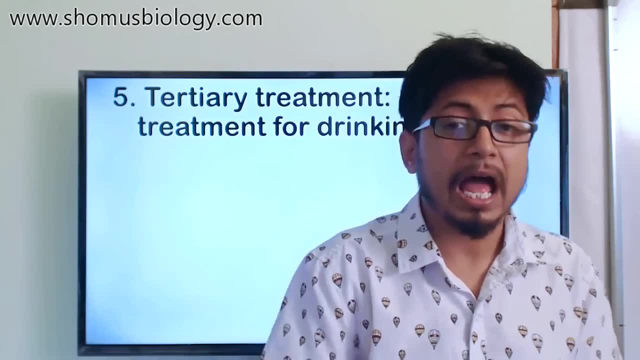 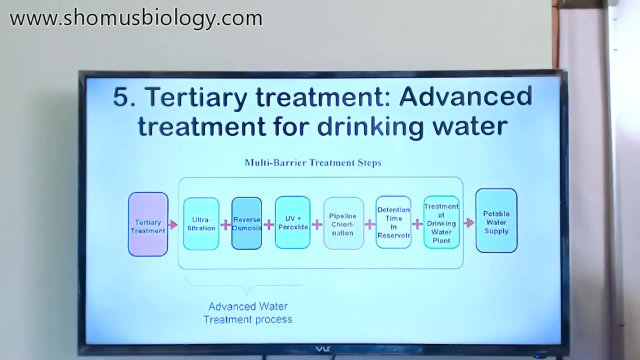 But in situations where the wastewater treatment at the end is destined to provide the water for drinking water purpose, Some additional features and safety are required. Even after tertiary treatment of wastewater, We take that water and that water can be used with multiple barriers of wastewater treatment. 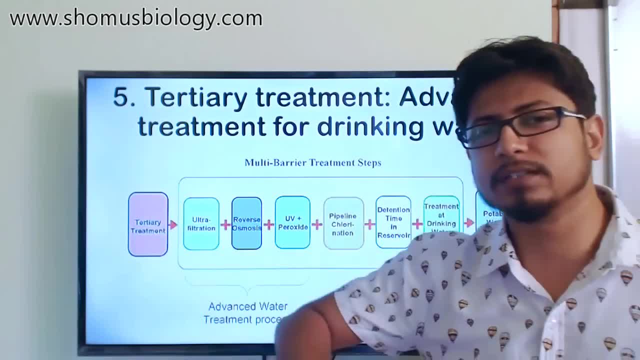 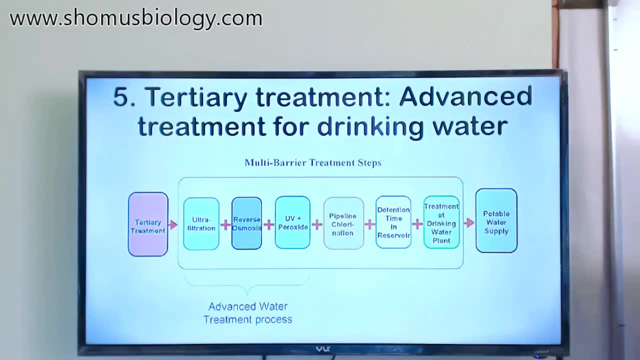 This. we cannot call it as a wastewater, Because at this point, after the water leaves the tertiary wastewater treatment plant, It's almost a pure water, But still we need to use some more substances, We need to take safety precautions before providing it for drinking. 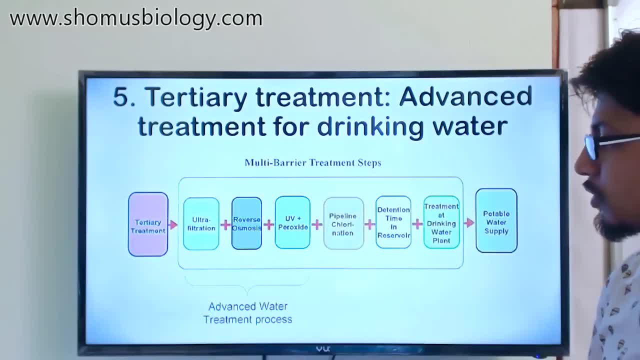 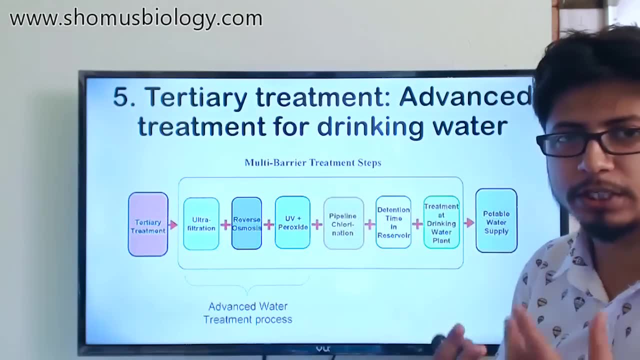 And that is involving ultrafiltration, or you can do reverse osmosis or UV radiation, or again chlorination in the pipe, Which is very cheap, and that's what generally done in India, Especially when chlorine is added to the municipal water pipe as well. From outside And treatment at drinking water plants, Because sometimes this water is transported from the wastewater, moves to drinking water plant. In the drinking water plant, the facility is a little different. They simply deal with all these modifications. Not all these modifications together is required. 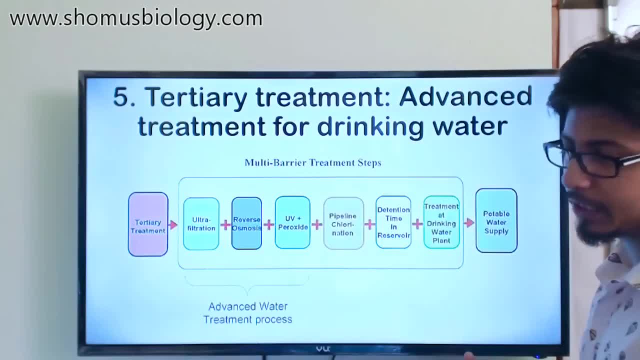 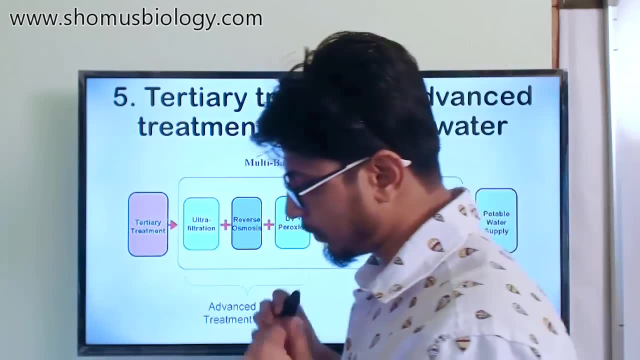 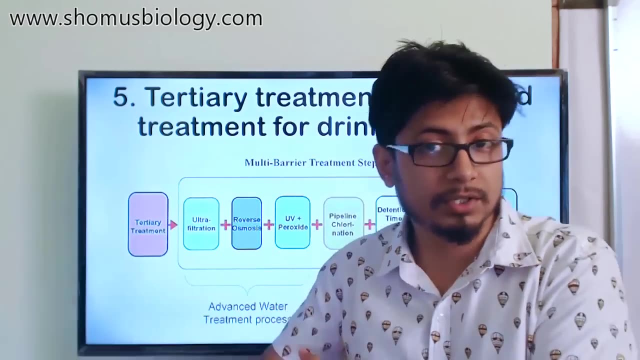 We simply need either reverse osmosis or UV or peroxide treatment or chlorination in the pipe, And then finally we transfer that water as a portable water supply to the household. So for the drinking water the treatment is little more advanced, even after the tertiary treatment.